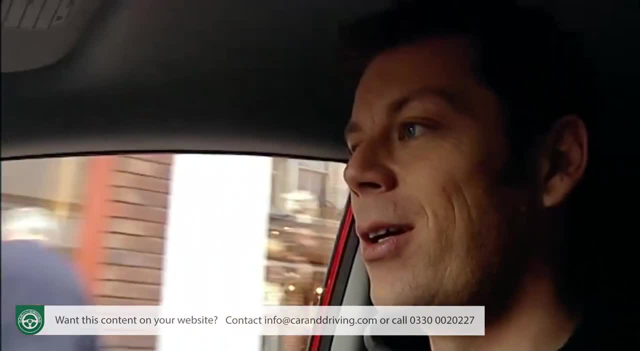 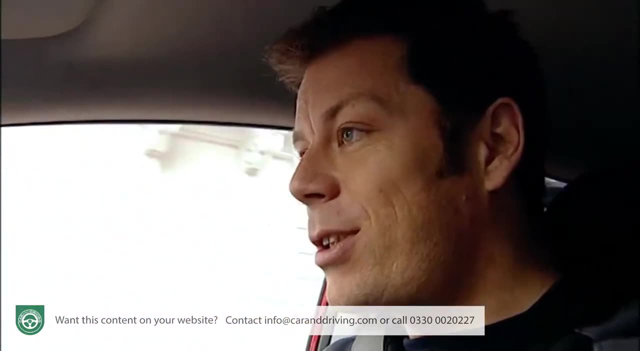 It's got a four-speed automatic, so you don't even have to worry about a clutch, and the turning circle is just ludicrously small, making the car very, very easy to park. What's a little bit disconcerting at times is quite how little car you have in front. 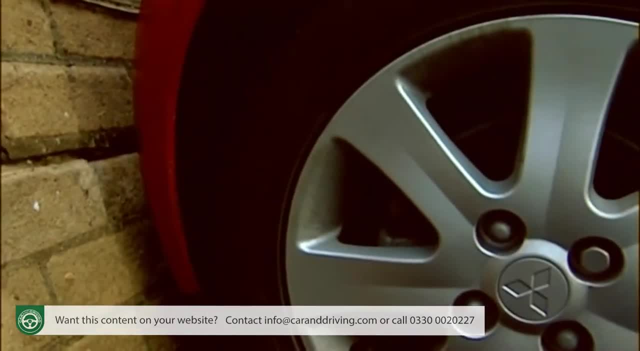 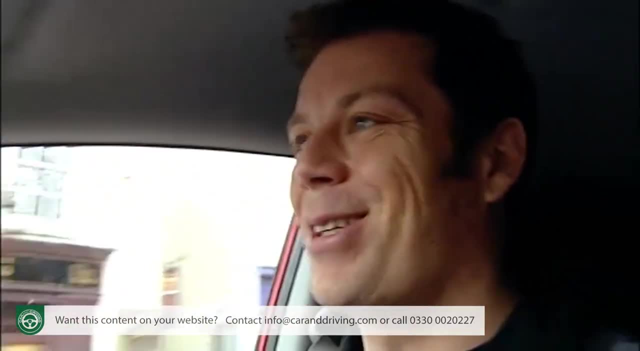 of you. When you pull up behind another vehicle in the traffic, it seems like you're almost climbing on board with them, But it makes a pretty decent noise as well. It's got a little turbo and it's as fast as it needs to be. 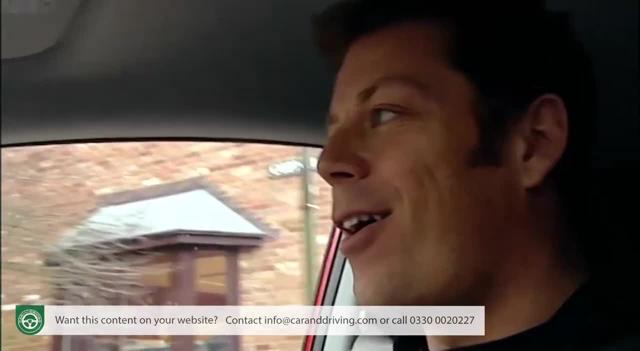 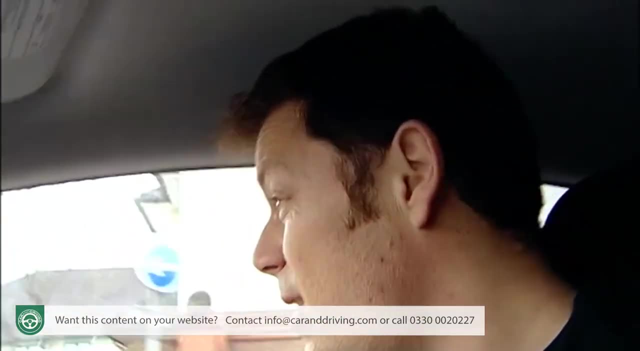 Rolls-Royce equations אלpiņš test drive. 112, now double theaves and stayed up easily during the last 40 minutes even on these cobbled roads here isn't too bad at all. It's a car that is a dedicated city car. You wouldn't want to subject it to long motorway journeys. 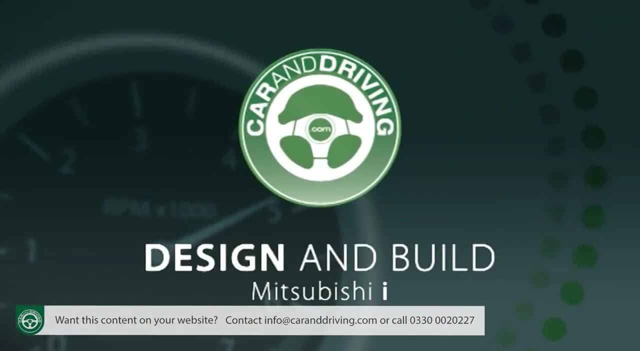 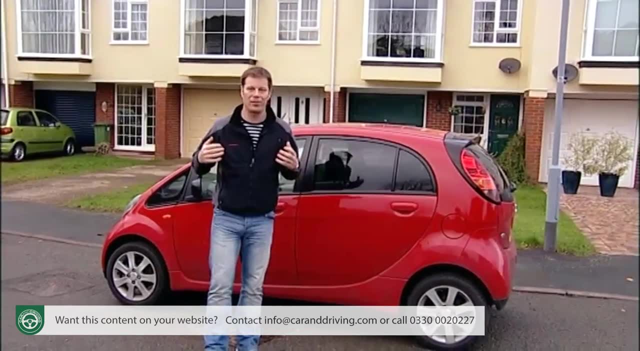 on a regular basis, but for what it does, it does its job very, very well. K-Kars: Where K-Kars have developed most significantly down the years is in space utilization. The old cars used to be tiny, You used to have to fold yourself into them, and the interiors 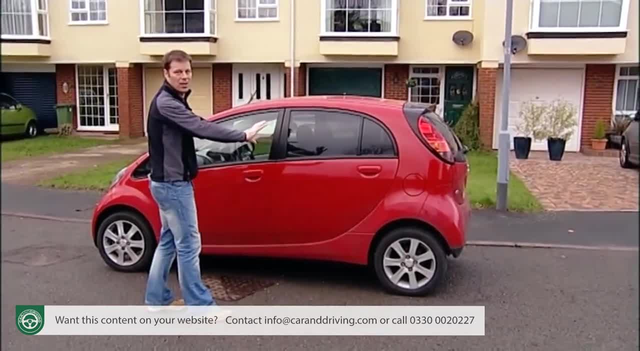 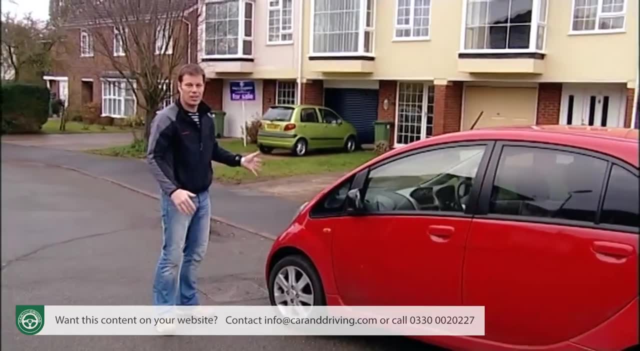 Now it's different. You look at this Mitsubishi i and the wheels are stretched out onto each corner, leaving lots of space inside the cabin. There aren't too many cars I can think of where the leading edge of the front tyre is actually in front of the headlamps. 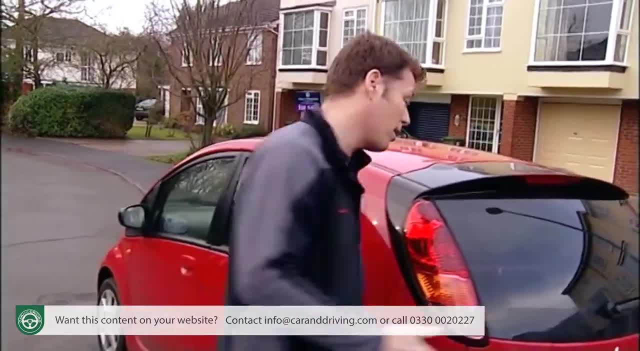 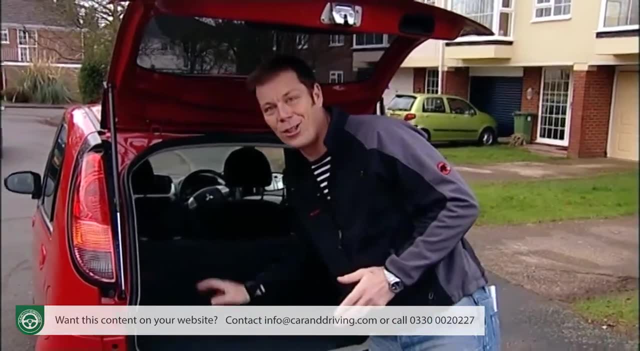 There's room inside for four adults. get one behind the other quite easily. There's even a usable boot. you can get the weekly shop in there, but the engine's under here, so don't leave your frozen goods in there too long, because it'll cook them. 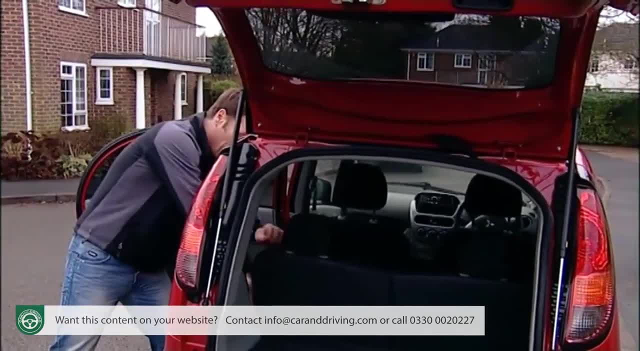 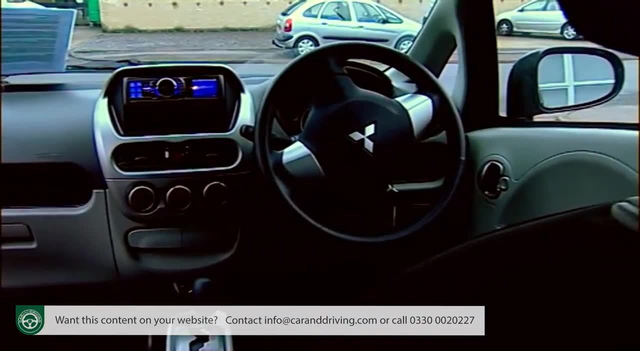 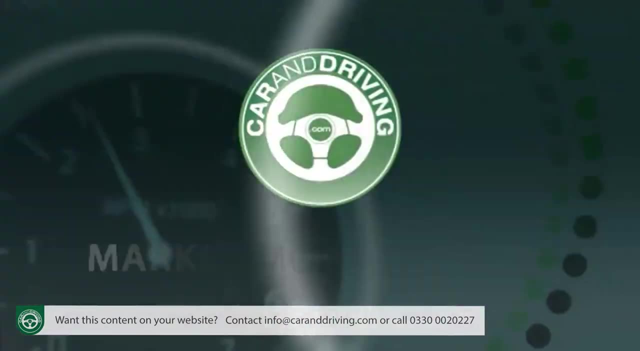 You can also fold the back seats down. both seats split so you can get longer items in there. It's a lot more versatile than its key rival, the Citycar Smart, by dint of having four seats and a much bigger boot area. You're probably wondering right now how you've managed down the years without OECOTEC's standard. 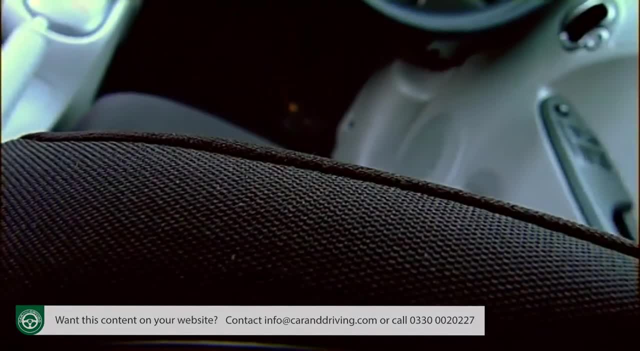 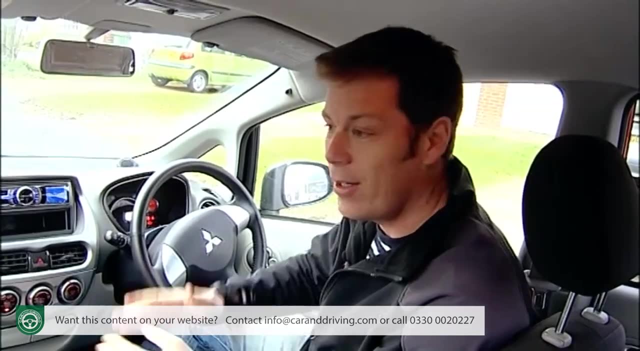 100 hyper-hylogenic seat fabric. I know I am this Mitsubishi. i comes with it as standard. It also comes with a new seat, which is a standard. It also comes with deodorising roof lining, so it smells as fresh as a daisy, even with me in here. 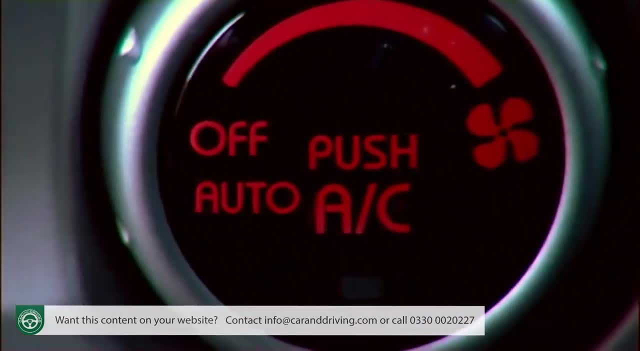 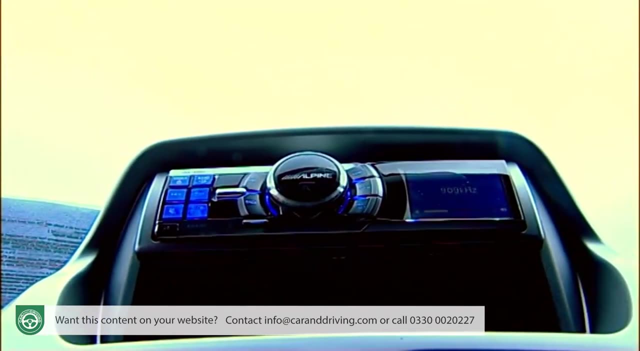 It's reasonably well equipped. you get climate controlled air conditioning, electric windows all round, anti-lock brakes and a CD stereo. This rather natty Alpine stereo is an optional extra. it's a bit punchier than the standard fit system which is integrated into the dash. 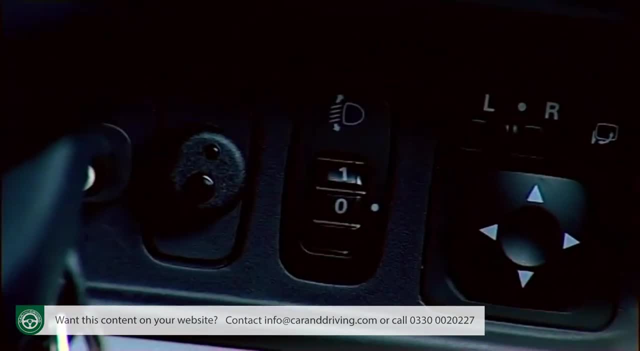 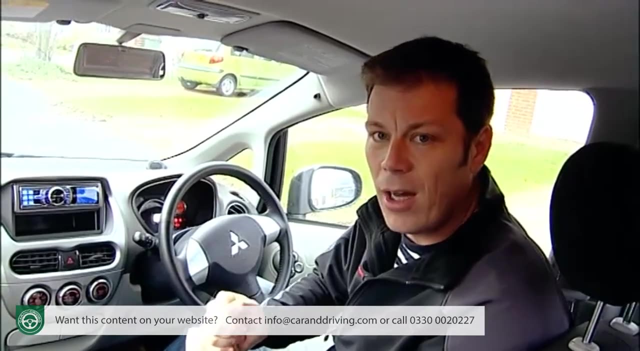 But aside from that it's a very, very well equipped car for the money, And if you look at the size of the automatic gearbox it starts to look a bit more competitive. Now there are a lot of rivals that cost about the same but are bigger cars. 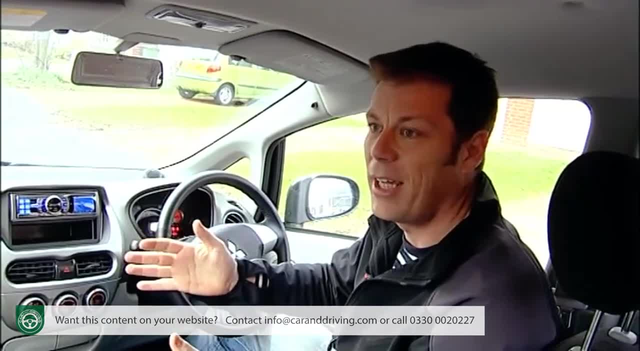 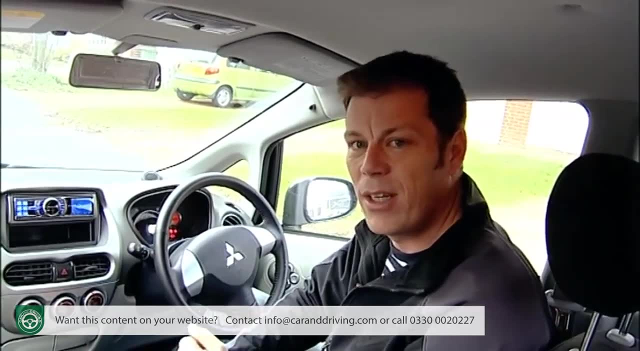 Cars like the Renault Clio, for example, And you're probably wondering why you should go for a tiny car like this that might be a bit out of its depth on the motorway, instead of one of these more versatile cars, And it's a good question. 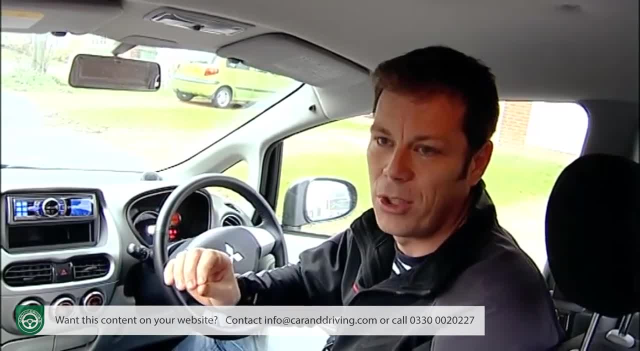 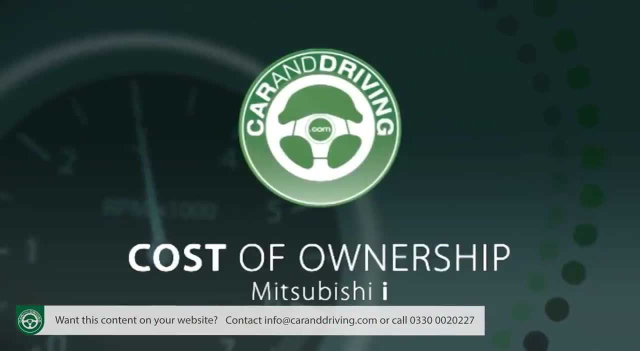 But Mitsubishi have realised that there are a core group of customers who aren't entirely price conscious and want a dedicated city car. that's different, does its thing in town better than anything else. The Mitsubishi i is one of the cheapest cars to run that it's possible to buy. 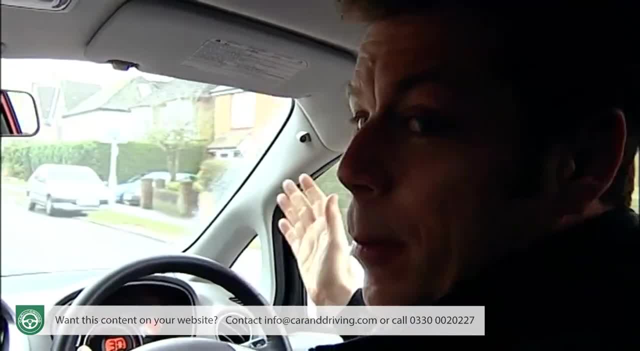 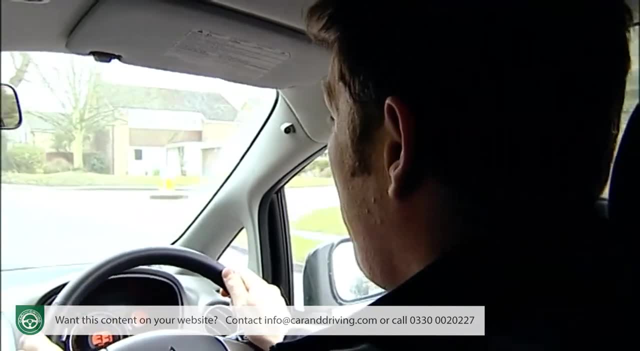 Limited supply means that the market's not going to be flooded with the things helping residual values, And the only possible caveat in that regard is if they do become quite popular and parallel importers start to bring them in in decent numbers. But I don't see that happening. 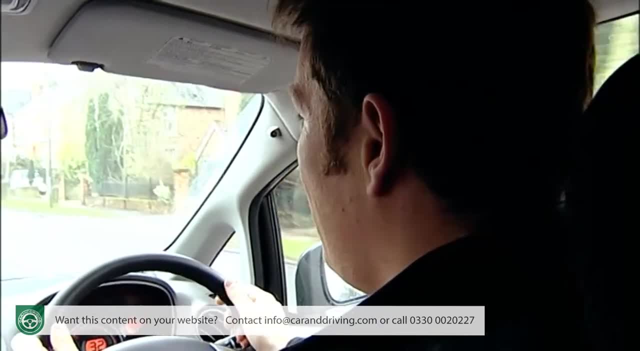 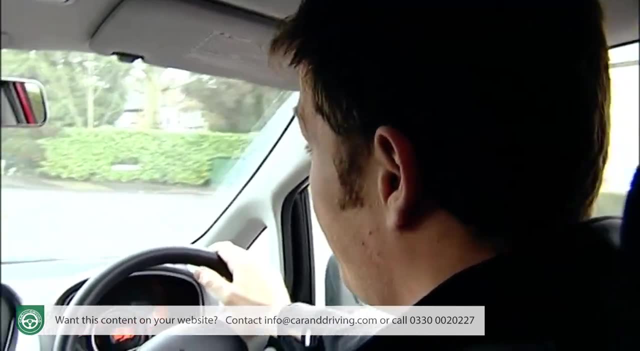 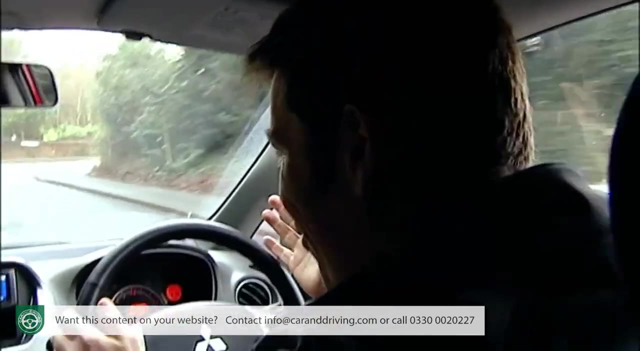 Emissions are super low. It's under 120 grams per kilometre, Which means it'll qualify for a very cheap road fund licence and also exemption from the London congestion charge. Fuel economy is about 55 miles per gallon, Although it does suffer a bit if you like to put your foot down. 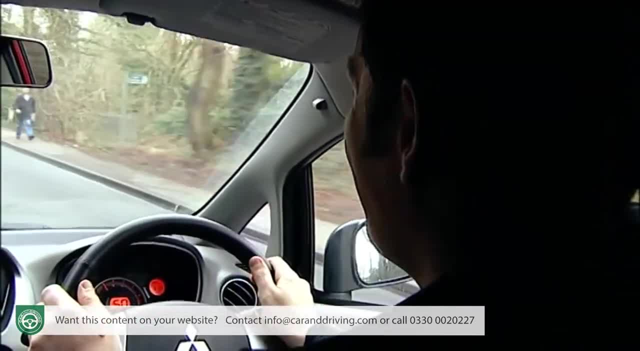 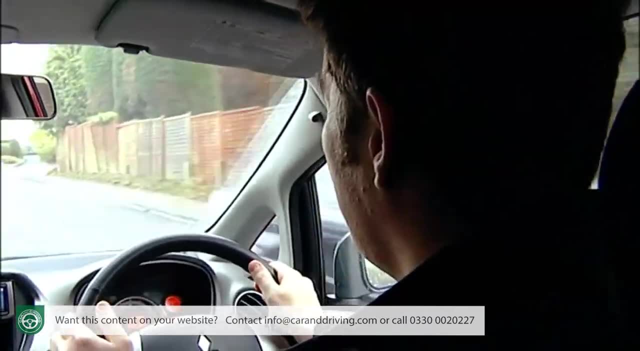 because this car does make quite a good noise and it's good fun to drive. Insurance is also very cheap, but security isn't quite as good as the best of the European cars. But other than that it's a very, very polished, all-round performance and a 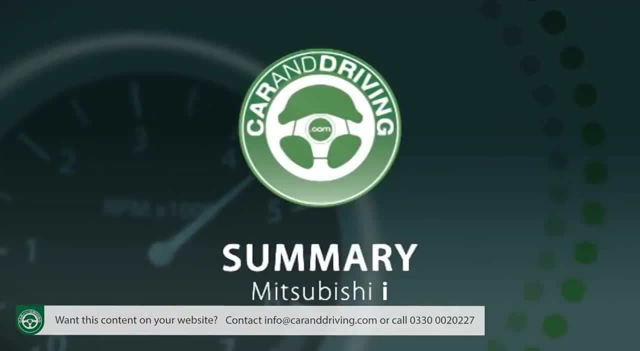 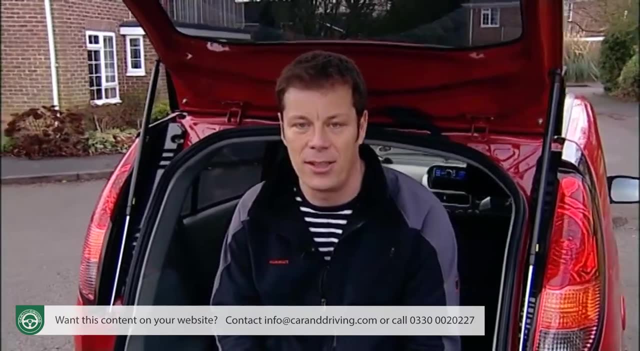 very cheap car to run. So if you're a 20 or 30 something and you're looking for the next small thing- Mitsubishi, i might well be it. Chances are that you've owned something like a Ford car, a Fiat Panda or a smart car. 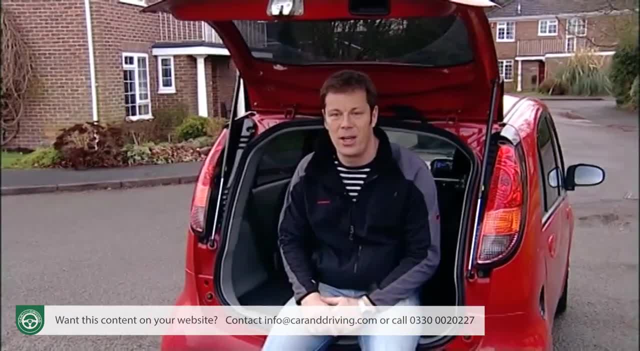 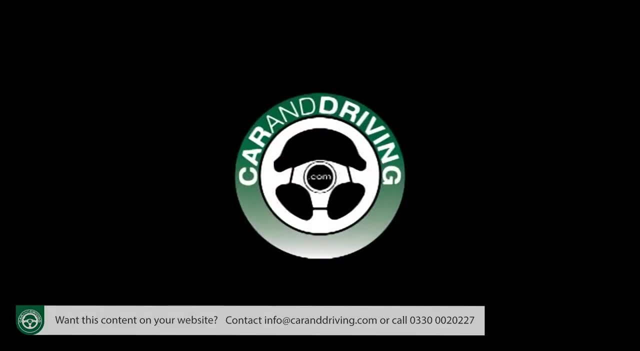 looking for something a bit different, a little bit more exotic. The Mitsubishi i certainly fits the bill. Drive one of these in city traffic and you'll definitely see the appeal.